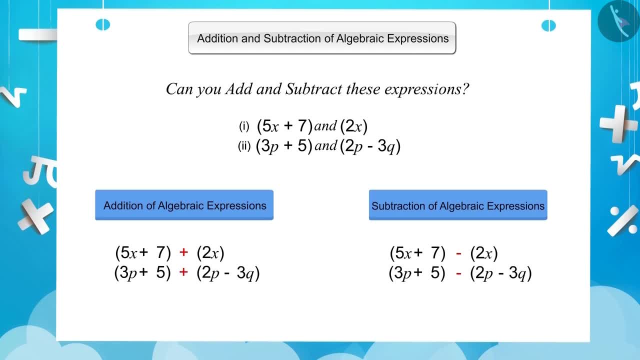 To understand these expressions, we must understand addition and subtraction of algebraic expressions. In our daily life, we use expressions and arithmetic operations in many situations. In this video we will learn how the algebraic expressions are added and subtracted. Example 1: 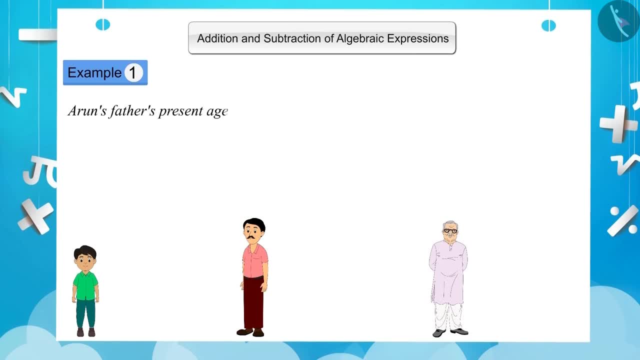 Arun's father's present age is twice Arun's age. If the age of Arun's grandfather is 3 years more than the sum of Arun's and his father's age, then how old is Arun's grandfather? Suppose Arun's age is a years? 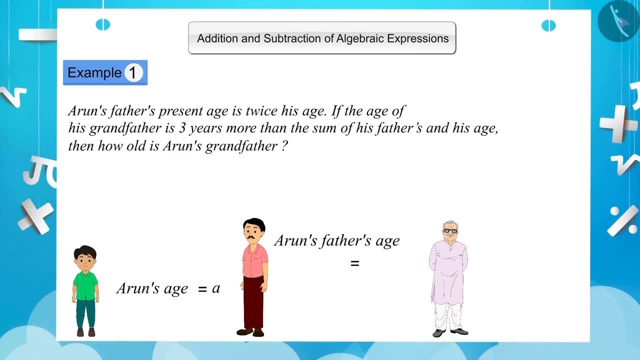 So Arun's father's age is equal to 2 times a, which is equal to 2a, As we know that Arun's grandfather's age is 3 years more than the sum of Arun's and his father's age. As we know that Arun's father's age is 3 years more than the sum of Arun's and his father's age. 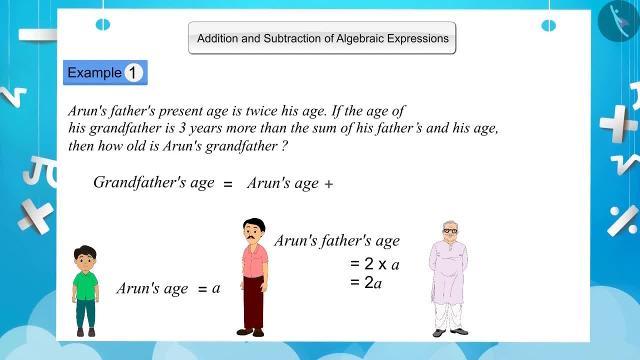 Grandfather's age is equal to Arun's age plus Arun's father's age plus 3, which is equal to a plus 2a plus 3. In this expression, a and 2a are like terms and 3 is an unlike term. 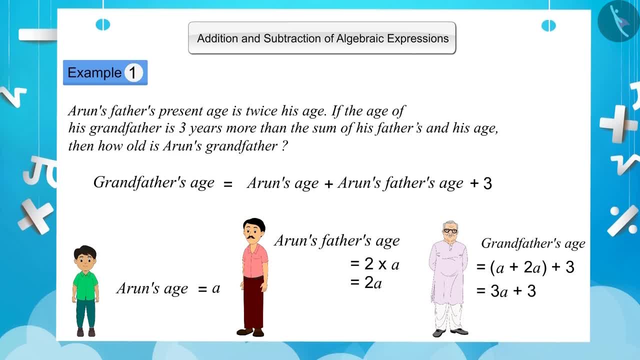 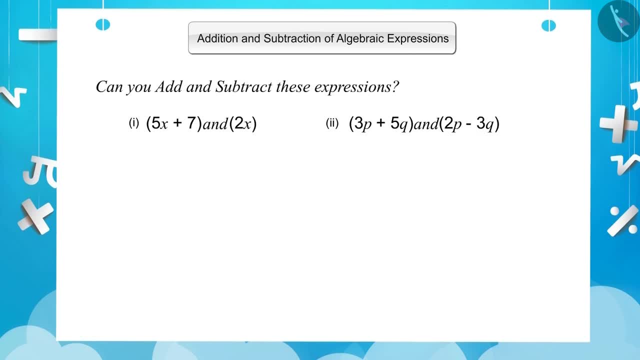 Now here we will add like terms and get 3a plus 3, which will be the age of Arun's grandfather, As we saw in some expressions earlier. 5x plus 7 and 2x and 3p plus 5q and 2p minus 3q. 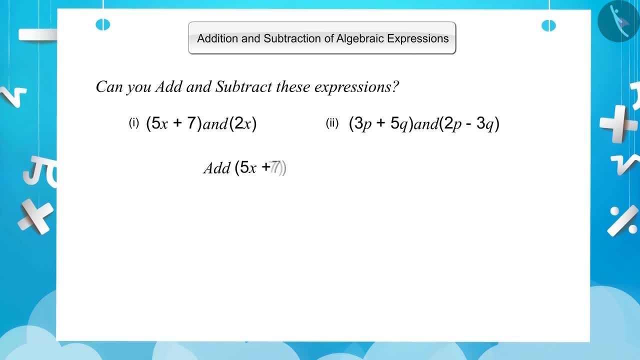 Now let's add and subtract them. Sum of 5x plus 7 and 2x. 5x plus 7 plus 2x: Here 5x and 2x are like terms, so we will arrange them as 5x plus 2x in brackets, plus 7. 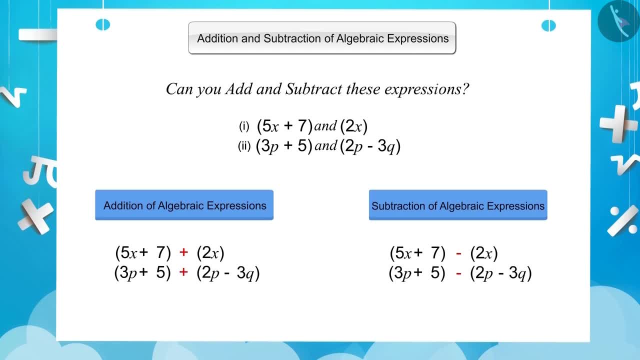 To understand these expressions, we must understand addition and subtraction of algebraic expressions. In our daily life, we use expressions and arithmetic operations in many situations. In this video we will learn how the algebraic expressions are added and subtracted. Example 1: 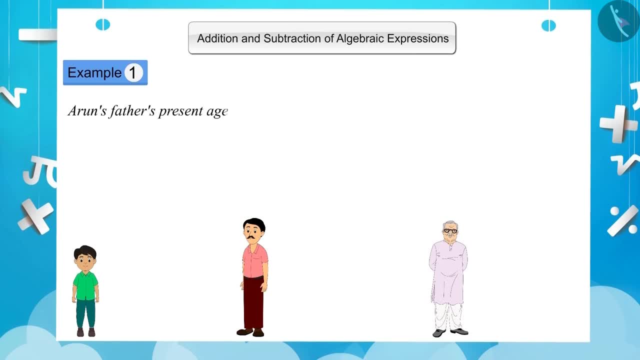 Arun's father's present age is twice Arun's age. If the age of Arun's grandfather is 3 years more than the sum of Arun's and his father's age, then how old is Arun's grandfather? Suppose Arun's age is a years? 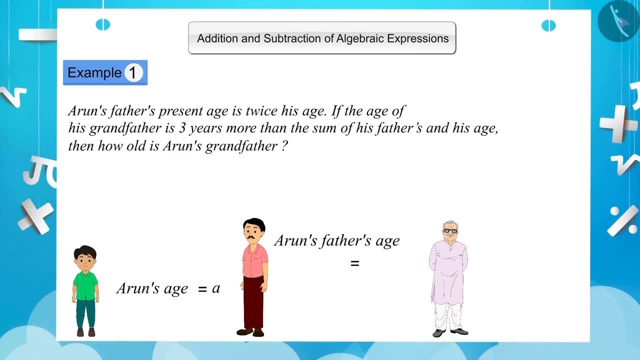 So Arun's father's age is equal to 2 times a, which is equal to 2a, As we know that Arun's grandfather's age is 3 years more than the sum of Arun's and his father's age. As we know that Arun's father's age is 3 years more than the sum of Arun's and his father's age. 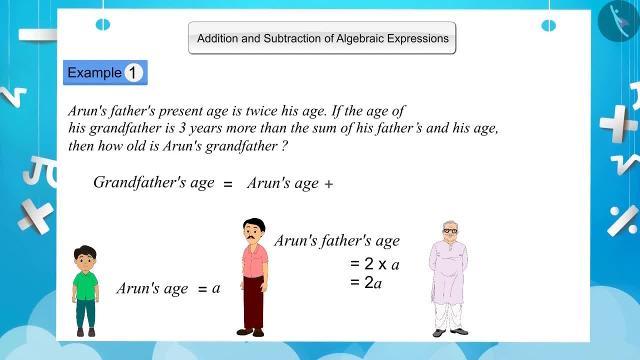 Grandfather's age is equal to Arun's age plus Arun's father's age plus 3, which is equal to a plus 2a plus 3. In this expression, a and 2a are like terms and 3 is an unlike term. 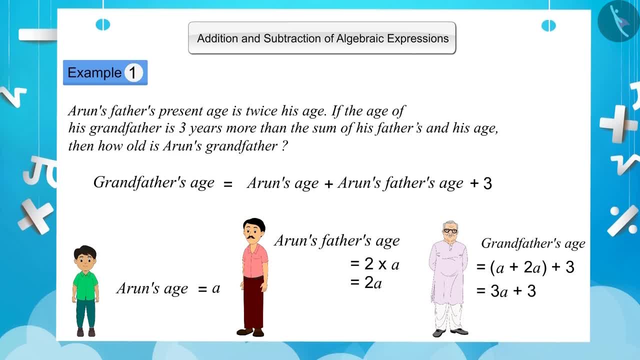 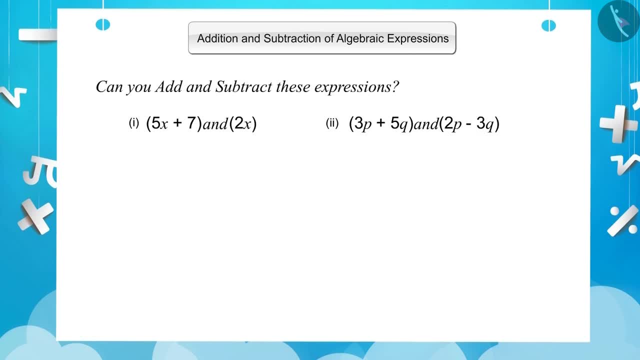 Now here we will add like terms and get 3a plus 3, which will be the age of Arun's grandfather, As we saw in some expressions earlier. 5x plus 7 and 2x and 3p plus 5q and 2p minus 3q. 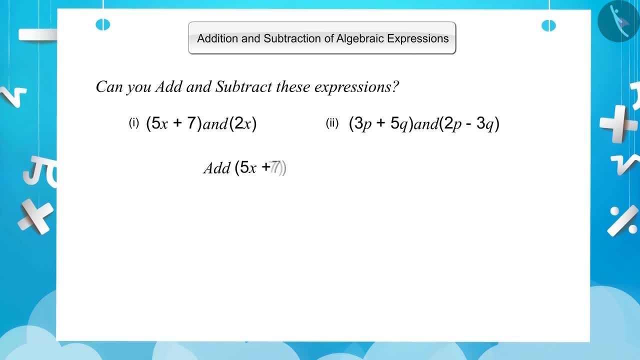 Now let's add and subtract them. Sum of 5x plus 7 and 2x. 5x plus 7 plus 2x: Here 5x and 2x are like terms, so we will arrange them as 5x plus 2x in brackets, plus 7. 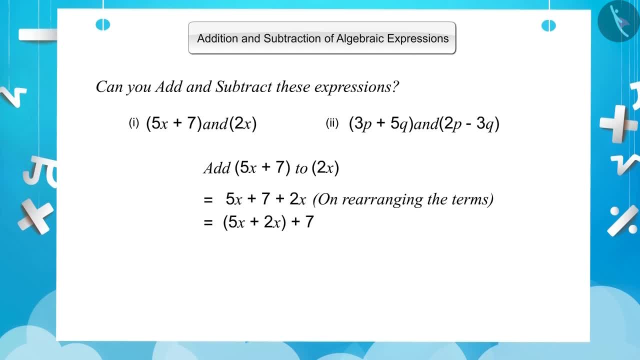 7 is the unlike term and will not be added. So by adding the like terms we get 7x plus 7, 5x plus 7 minus 2x. Here 5x and 2x are like terms, so we will rearrange these two terms. 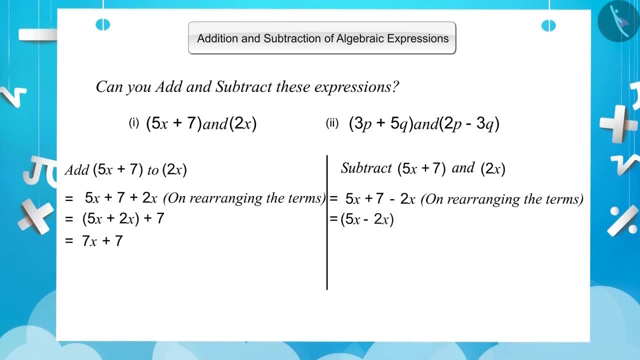 That is 5x minus 2x, in brackets plus 7. 7 is the unlike term and hence cannot be subtracted. Therefore, by subtracting the like terms we will get 3x plus 7.. Sum of 3p plus 5q and 2p minus 3q. 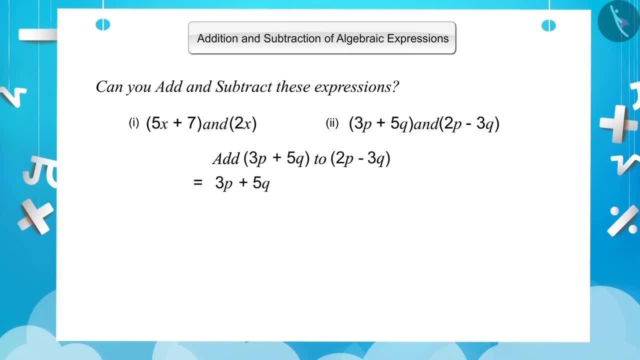 3p plus 5q plus 2p minus 3q. Here 3p and 2p and 5q and 3q are like terms, So we can rearrange it to get the like terms together: 3p plus 2p in brackets plus 5q minus 3q in brackets. 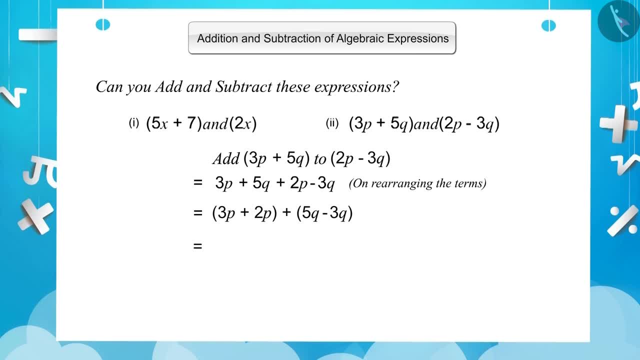 By combining the like terms, we get 5p plus 2q, 3p plus 5q minus 2p plus 3q. Subtraction of 3p plus 5q and 2p plus 3q: 3p plus 5q and 2p minus 3q. 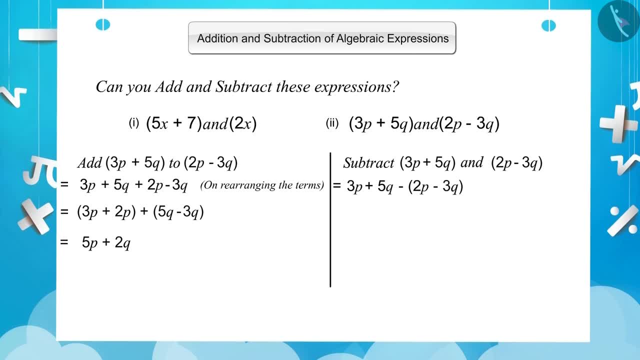 Here we will bring the terms out of the brackets: 3p plus 5q minus 2p plus 3q. As we know that, in subtraction, while eliminating the brackets, the sign of those terms inside the bracket changes 3p plus 5q minus 2p plus 3q. 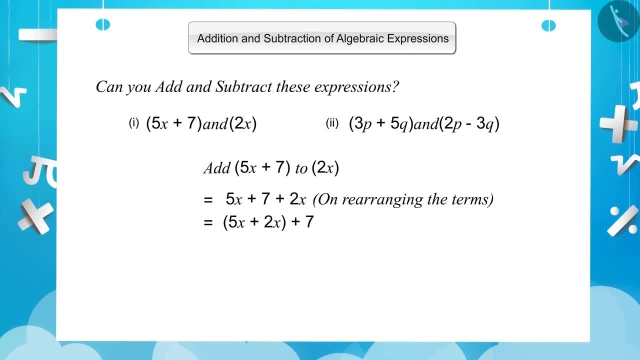 7 is the unlike term and will not be added. So by adding the like terms we get 7x plus 7, 5x plus 7 minus 2x. Here 5x and 2x are like terms, so we will rearrange these two terms. 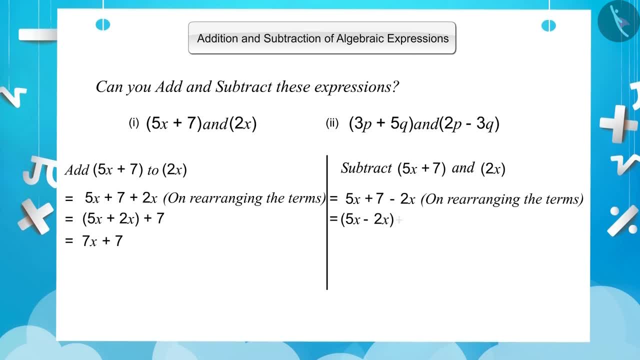 That is 5x minus 2x, in brackets plus 7. 7 is the unlike term and hence cannot be subtracted. Therefore, by subtracting the like terms we will get 3x plus 7.. Sum of 3p plus 5q and 2p minus 3q. 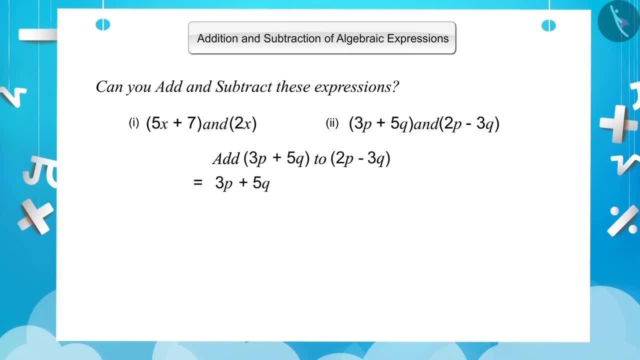 3p plus 5q plus 2p minus 3q. Here 3p and 2p and 5q and 3q are like terms, So we can rearrange it to get the like terms together: 3p plus 2p in brackets plus 5q minus 3q in brackets. 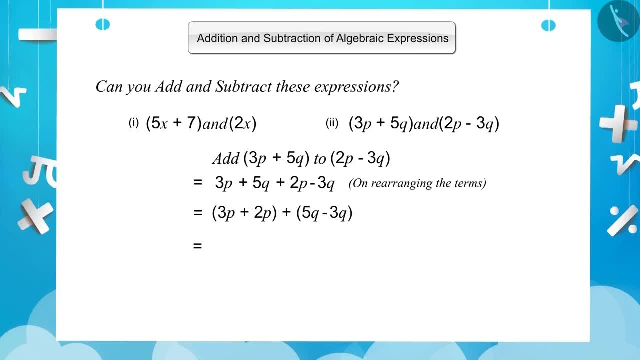 By combining the like terms we get 5p plus 2q, 3p plus 5q minus, 2p plus 3q. Subtraction of 3p plus 5q and 2p minus 3q. Here we will bring the terms out of the brackets. 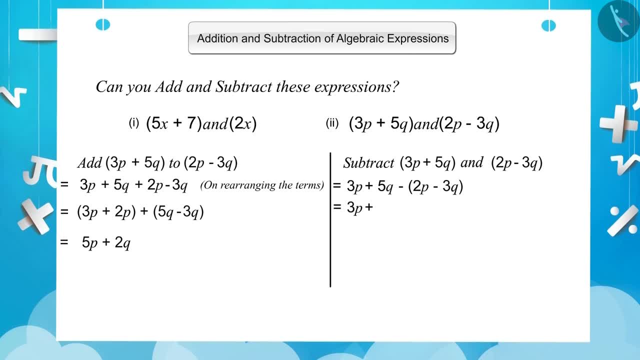 As we know that in subtraction, while eliminating the brackets, the sign of those terms inside the bracket changes 3p plus 5q minus 2p plus 3q. Here 3p and 2p and 5q and 3q are like terms. 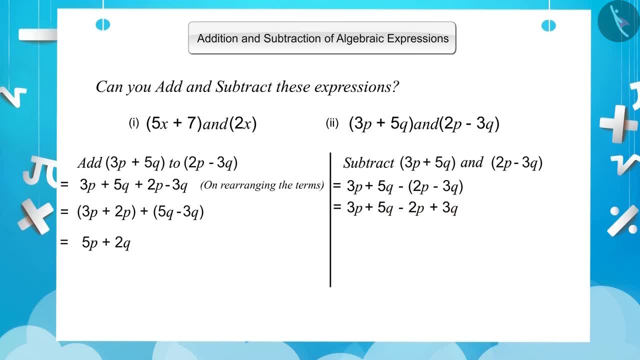 Here 3p and 2p and 5q and 3q are like terms, So we will rearrange the like terms 3p minus 2p in brackets plus 5q plus 3q in brackets. By combining the like terms we will get 1p plus 8q. 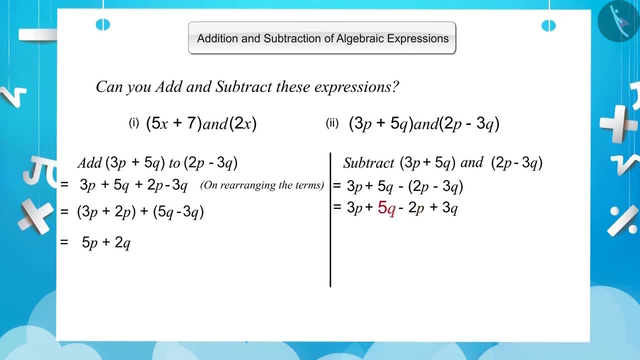 Here 3p and 2p and 5q and 3q are like terms, Here 3p and 2p, and 5q and 3q are like terms, So we will rearrange the like terms.